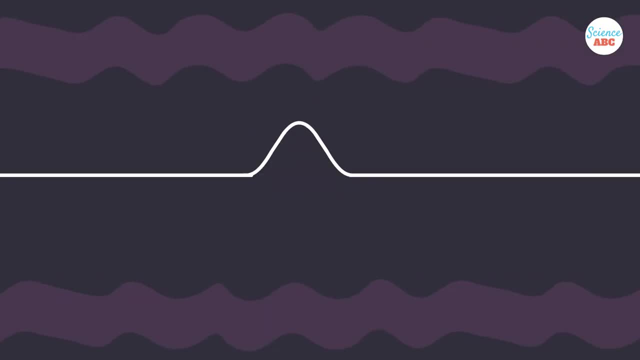 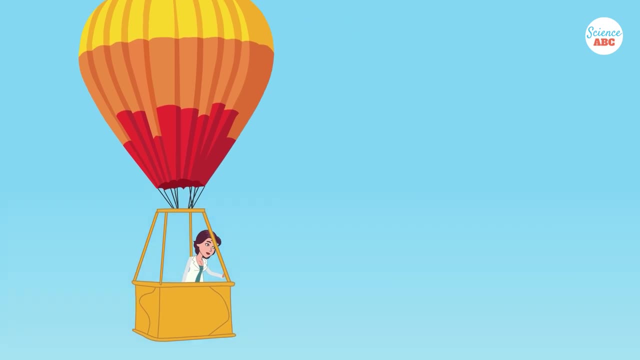 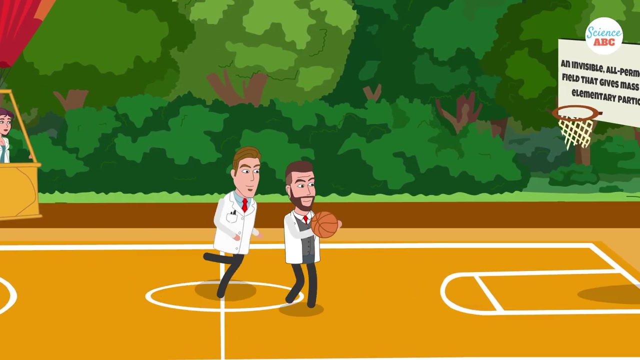 This theory argues that every particle can be represented by a wave in its corresponding field. In the year 1964, Peter Higgs, Francois Englert and four other scientists proposed a rather unique idea to explain why certain particles had mass. They hypothesized that the entire universe is 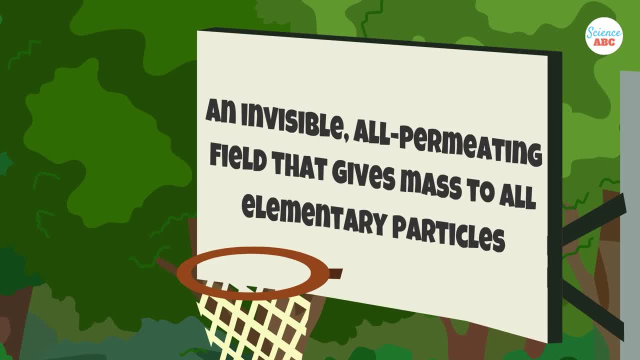 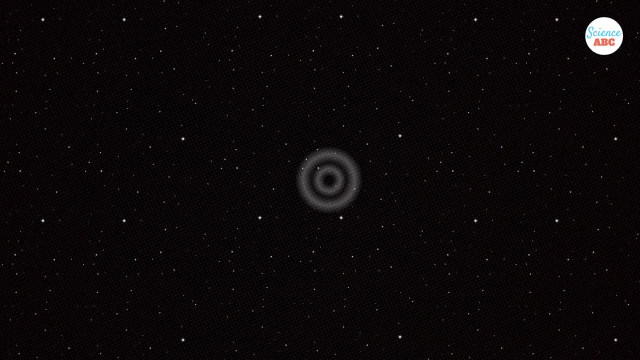 filled with an invisible, all-permeating field which gives mass to all elementary particles. The field in question is called the Higgs field. A wave, ripple or disturbance in that field is therefore called the Higgs boson or the Higgs particle. This theory 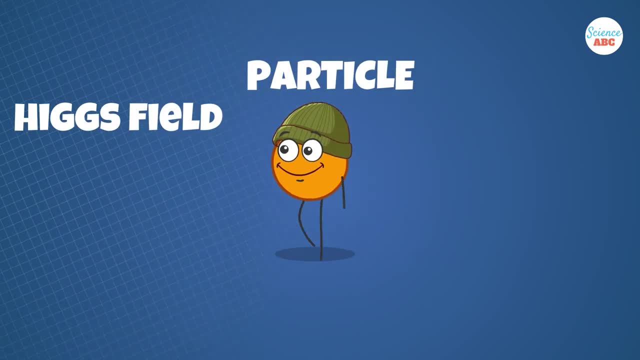 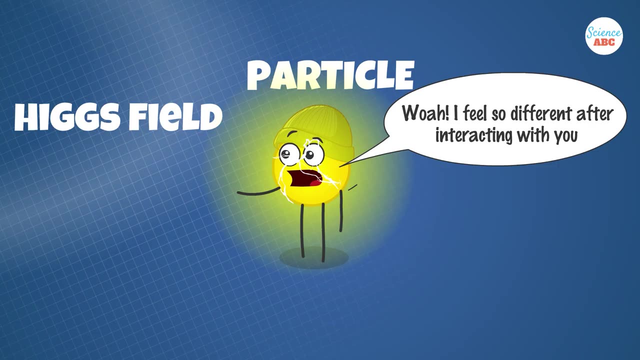 suggests that particles do not have a mass of their own. Rather, they get their mass by interacting with the Higgs field. How heavy a particle is will be determined by how strongly a particle interacts with the Higgs field: Electrons, quarks and other elementary particles. 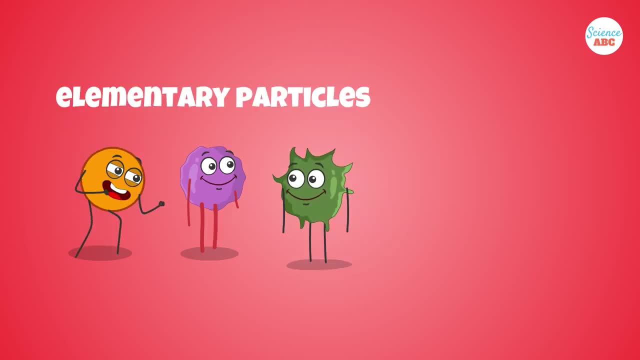 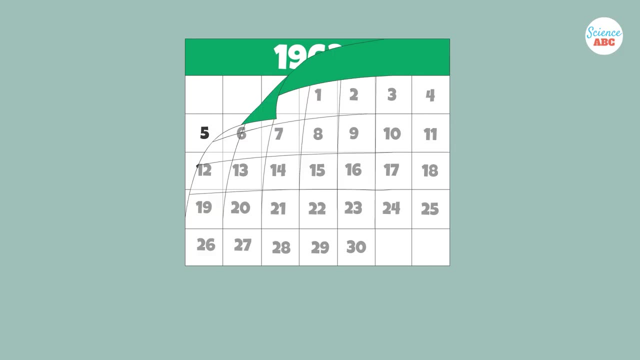 however, do not interact with the Higgs field in different ways and therefore have different masses. Photons, however, do not interact with the field and thus have no mass. Now remember, the existence of the Higgs field was just an idea proposed in 1964 by a few. 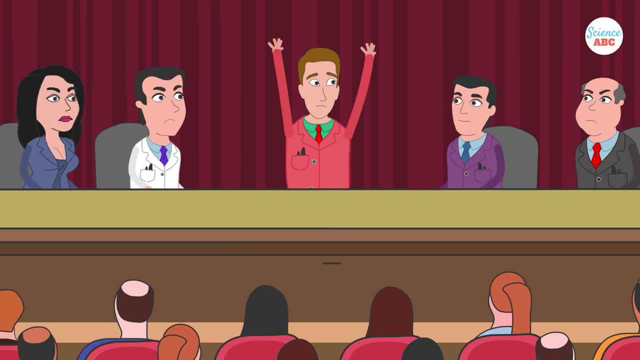 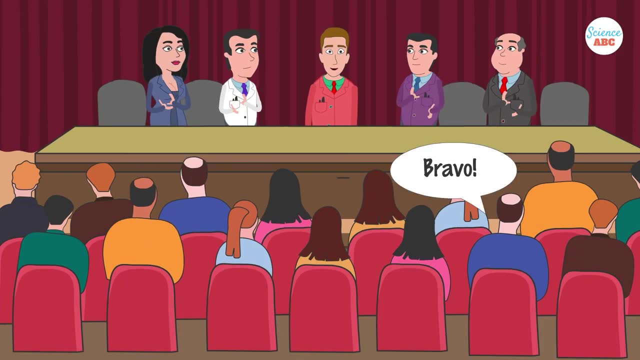 scientists. After initially facing skepticism from the scientific community, the idea was later hailed as a brilliant one. However, for many years, it was exactly that, just an idea. No proof for this field existed. All of that changed on July 4th 2001,, when 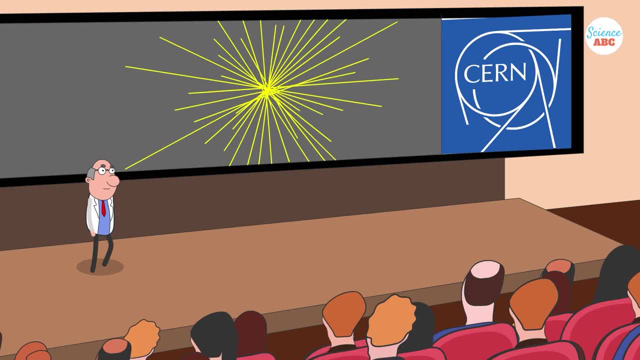 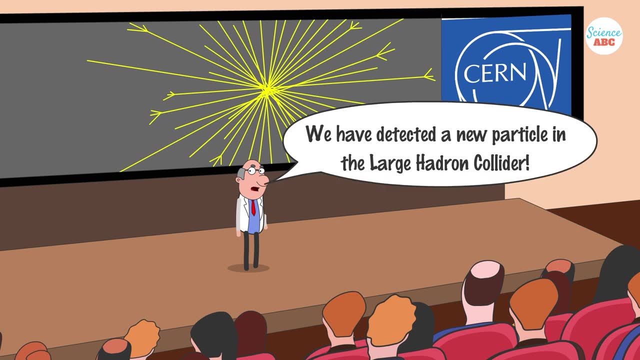 the Higgs field was discovered. The Higgs field was discovered by a group of scientists, and it was in 2012 when researchers at CERN confirmed the existence of this mass-giving field because a new particle, the Higgs boson, had been discovered in the Large Hadron Collider. 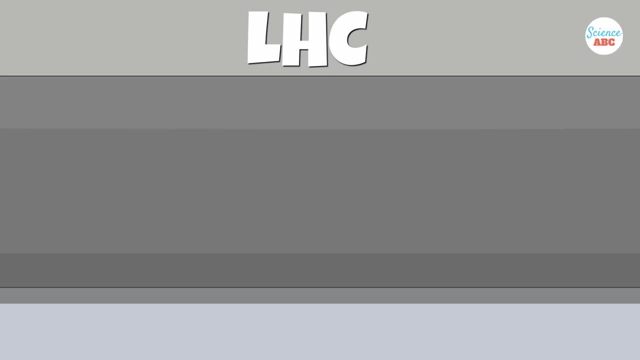 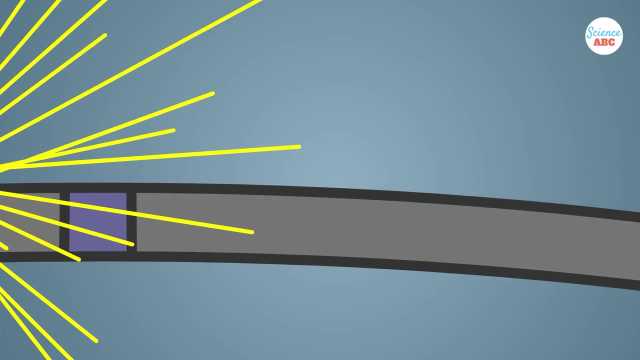 the largest and most powerful particle accelerator in the world. The LHC accelerates protons and charged ions at a speed close to the speed of light and then smashes them against another beam of elementary particles. This collision produces massive particles and the Higgs. 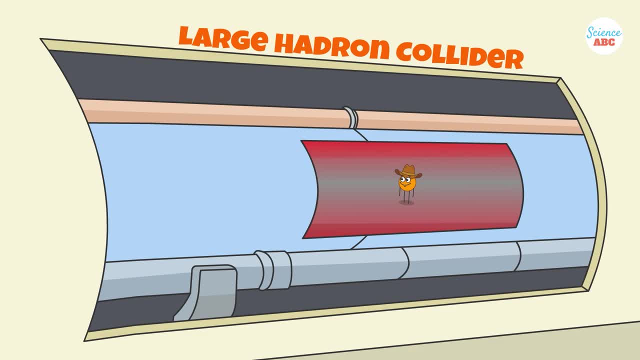 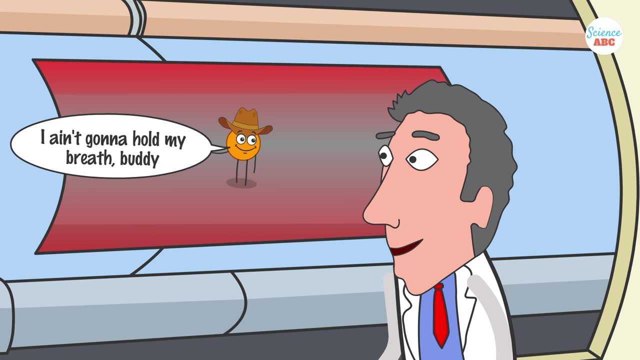 boson is one of them. Unfortunately, the Higgs boson doesn't sit around for long. In fact, it decays into smaller particles almost as soon as it's detected. That's why it is so difficult to detect massive particles like the Higgs boson To understand.